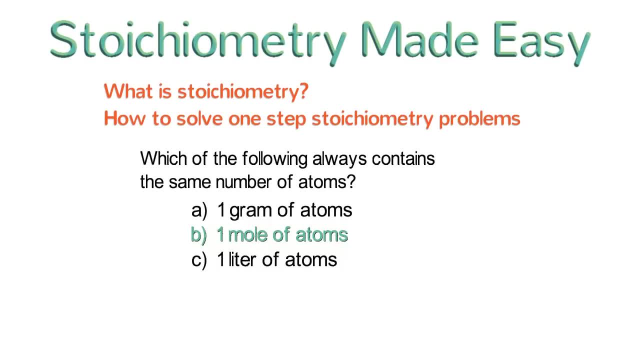 The correct answer is B 1 mole of atoms, which is equal to 600 billion trillion atoms. Remember that, just like a dozen is 12 things, a mole is simply a very large number of things And because the mole refers to the number of things, we will need to use the mole extensively when we do stoichiometry. 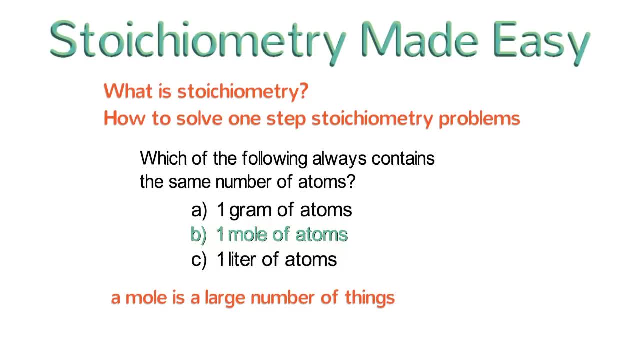 So what in the world is stoichiometry? The word comes from two Greek roots: stoikion, which means element, and metron, which means measure. Basically, stoichiometry is a scientist's way of measuring elements and other chemicals in a chemical reaction. 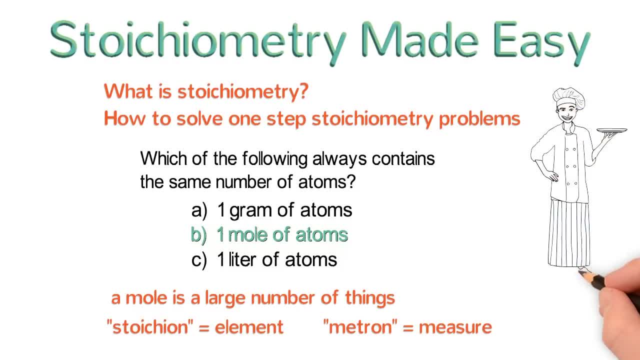 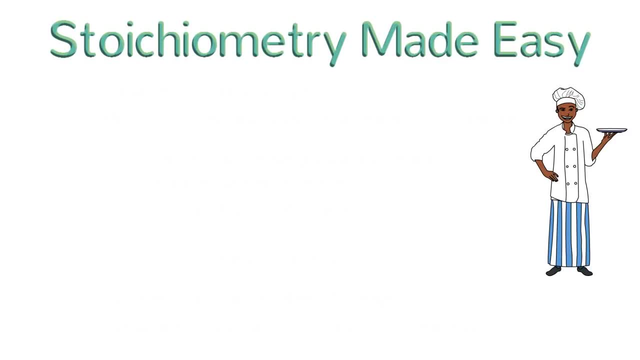 It's a lot like the way a chef measures the ingredients. In fact, chemistry is a lot like cooking. Imagine for a second that you're home alone and craving some grilled cheese sandwiches, but you don't know how to make one. So you call up your friend and say: 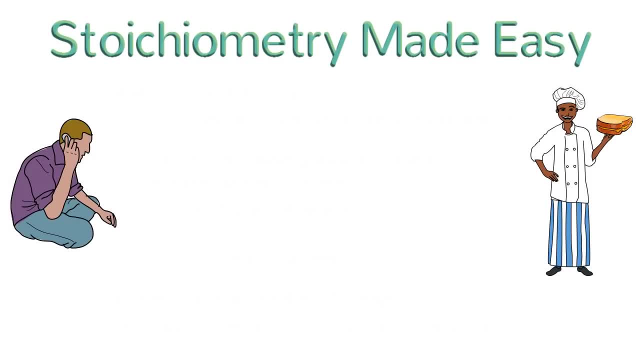 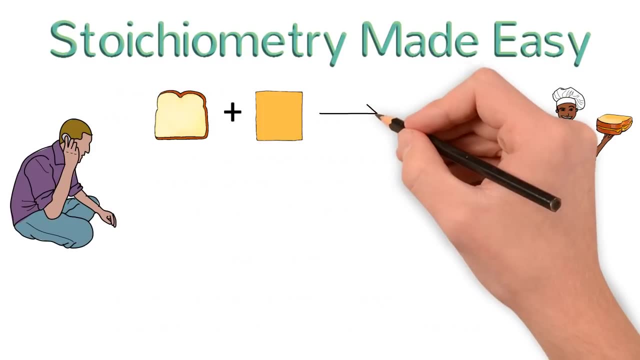 Hey man, how do you make a grilled cheese sandwich? And he says: Dude, chill, It's real easy. Just take some bread, put some cheese in the middle, heat it up and you got yourself some grilled cheese. How much bread, How much cheese? you ask. 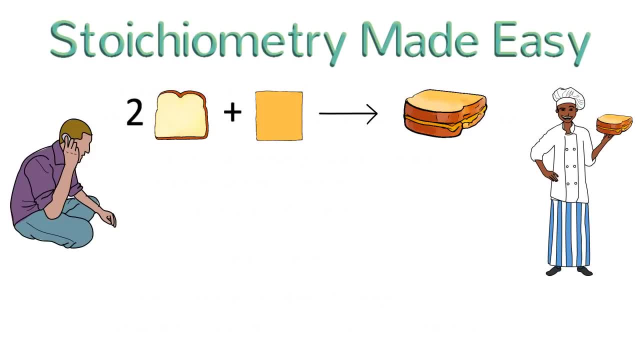 Two slices of bread and one slice of cheese. One slice of cheese is all you need to make one sandwich. So there you go. You've got your recipe. In chemistry, the recipe is the balanced chemical equation. So where does stoichiometry come in? 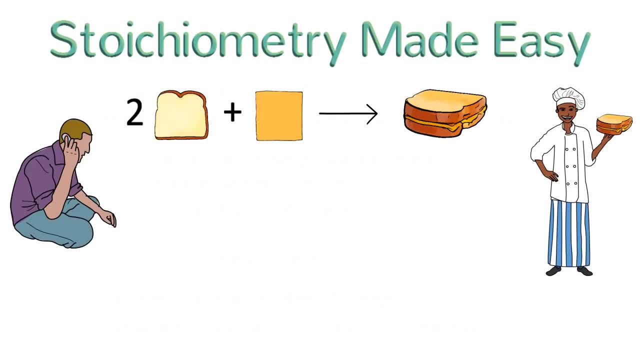 Let's suppose you are super hungry and you want to make seven grilled cheese sandwiches. You need to know how much of each ingredient to use. Let's start with the first ingredient. How many slices of bread do you need to make seven grilled cheese sandwiches? 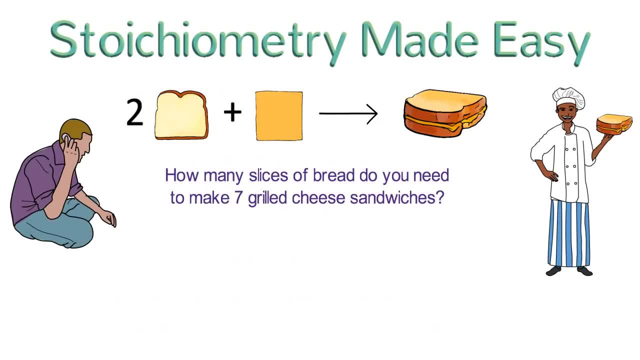 You can probably solve this in your head, but please follow the logic of my method In order to solve this problem. we are first going to write down the quantity that we know: Seven grilled cheese sandwiches. Next, we are going to multiply this by the ratio of bread to sandwiches. 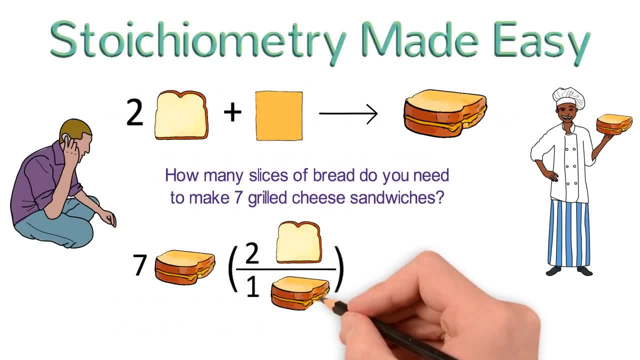 You need two slices of bread to make one sandwich. Where did I get those numbers? The recipe, or the balanced equation, tells us the ratio of the ingredients and products. Bread and sandwiches are in a two to one ratio. We put the two slices of bread on top because that is what we are solving for. 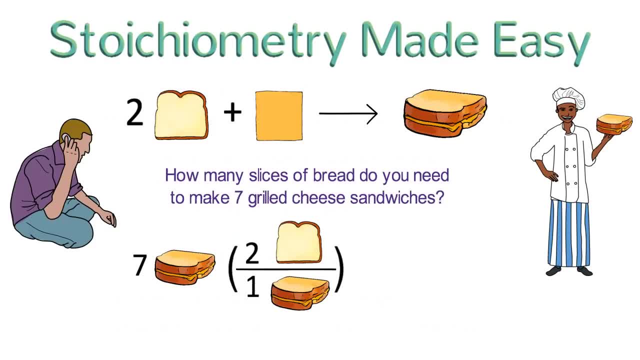 and the one sandwich on the bottom, because that is the quantity that we started with. Sandwiches on the top and bottom cancel each other out and we are left with seven times two slices of bread to make fourteen slices of bread, which is our final answer. 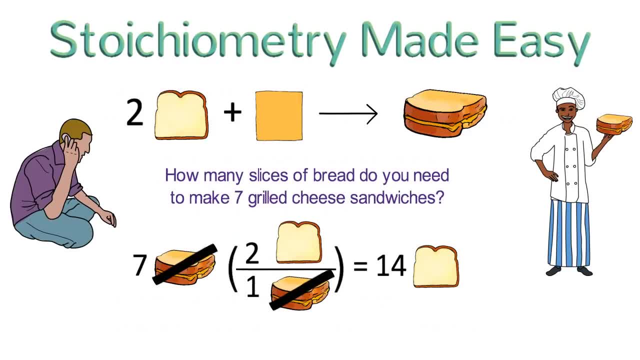 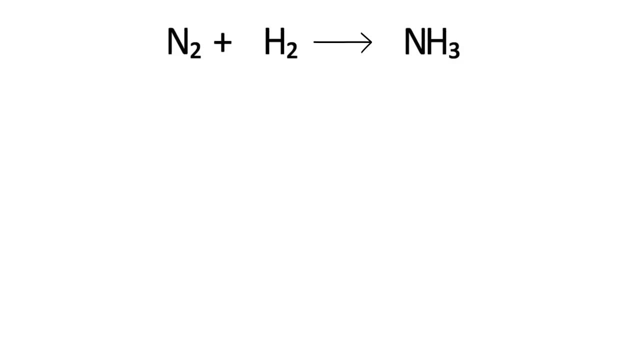 Notice that this is really a unit conversion problem and the balanced equation is our conversion factor. Okay, now we are going to do the exact same thing with chemicals that we just did with food. Check out this reaction: Nitrogen reacts with hydrogen to produce NH3, which is called ammonia. 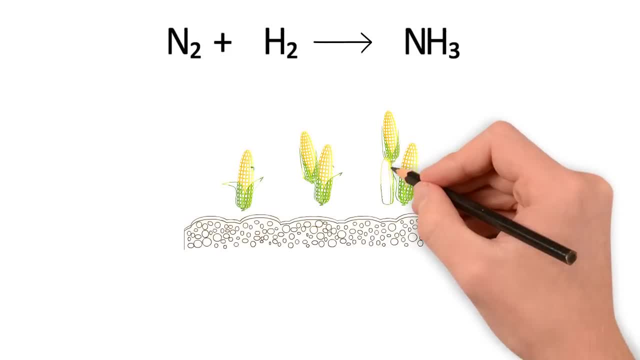 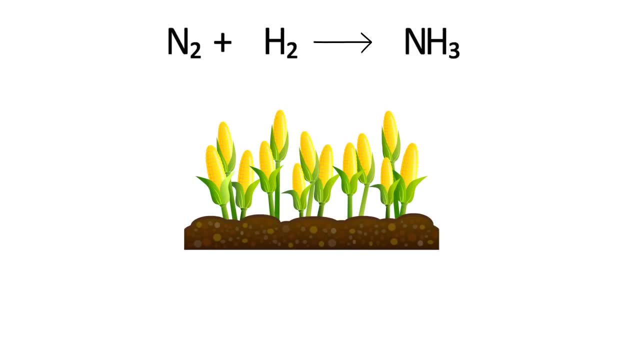 This reaction is known as the Haber process, which is primarily used to make fertilizer. Fertilizer helps crops grow and becomes part of our food. In fact, more than half of the nitrogen in your body probably comes from this reaction, so it is pretty important. 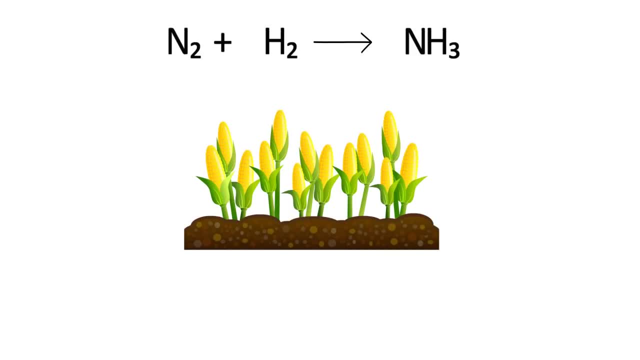 As it is written, the reaction is not balanced. There are two nitrogens on the left and only one on the right, so we put a two in front of ammonia to balance the balance. This gives us six hydrogens on the right side but only two on the left. 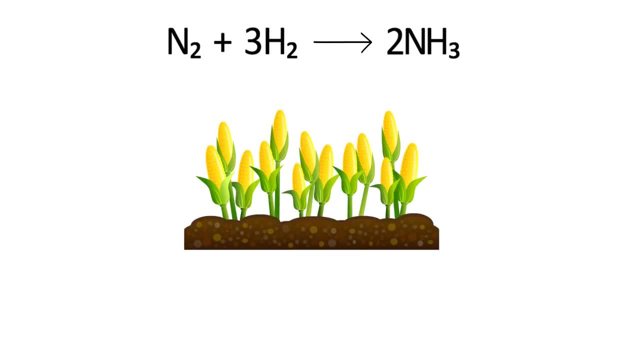 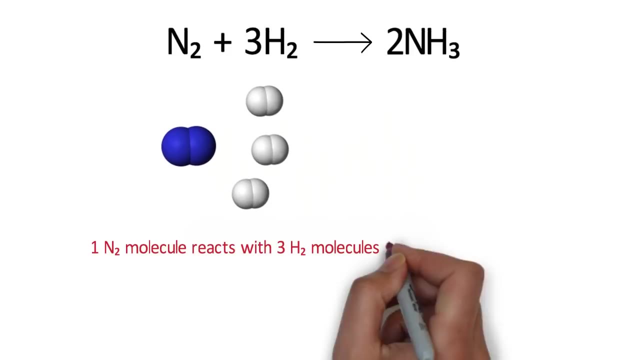 so we put a three in front of hydrogen. Now the reaction is all balanced. Remember, our balanced reaction is a recipe. so what is it actually telling us? The balanced chemical equation tells us that one nitrogen molecule reacts with three hydrogen molecules to make two ammonia molecules. 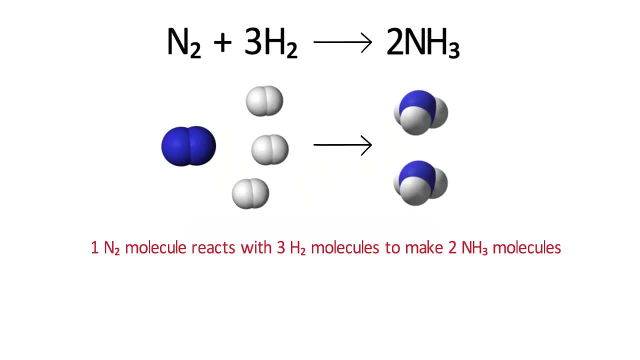 Well, what if we have more? Let's say we have ten nitrogen molecules, How many hydrogen molecules would they react with? That's right, thirty, And the reaction would produce twenty ammonia molecules. The balanced chemical equation tells us that nitrogen, hydrogen and ammonia 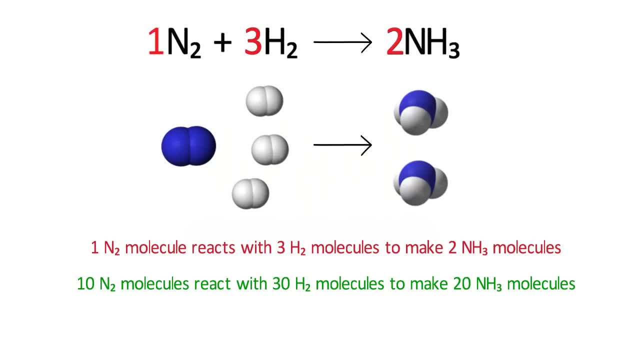 are always in a one to three to two ratio, no matter how big or small the reaction is. So let's talk about a large amount of nitrogen. The air you breathe in every minute when you are walking contains approximately six hundred billion trillion nitrogen molecules. 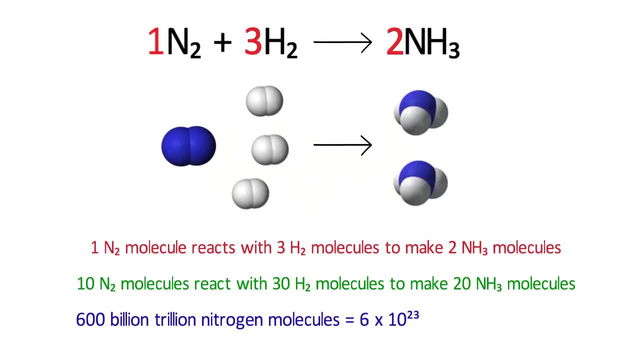 Which is equal to six times ten to the twenty-third. Does that number look familiar? Yes, we're talking about one mole of nitrogen, And one mole of nitrogen will react with three moles of hydrogen to make two moles of ammonia. Where am I getting those numbers? 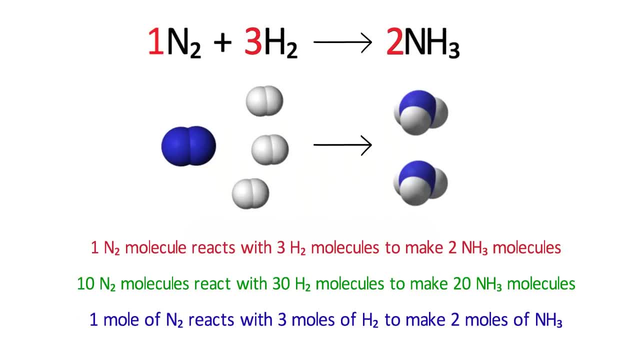 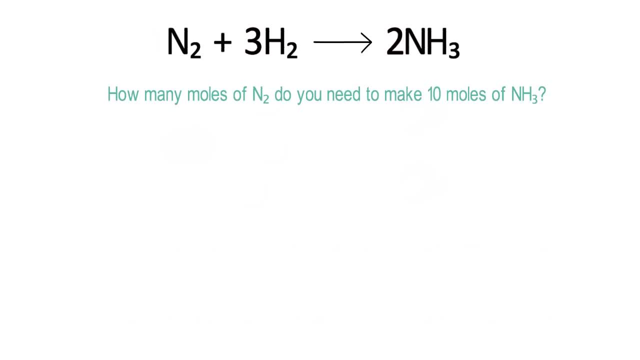 They are the big numbers in front of the chemicals in the balanced reaction. Let's try a sample problem. How many moles of nitrogen do you need to make ten moles of ammonia? First write down the quantity that you know: Ten moles of ammonia. 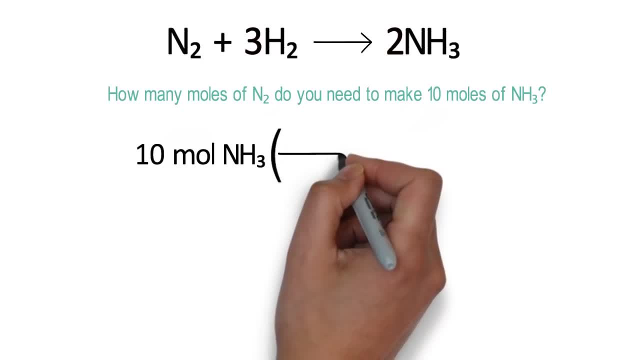 Next, multiply that by the ratio of nitrogen to ammonia in the balanced reaction. Since we are starting the problem with ammonia, we put the two NH3 on the bottom. This two NH3 comes directly from the balanced reaction. Because we are solving for nitrogen, we put one N2 on the top. 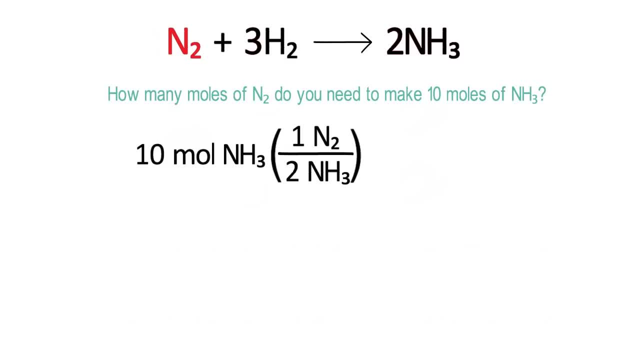 That one. N2, also comes from the balanced reaction. Remember, if no number is written in front of a chemical, that means the coefficient is one. So I'll do the fraction. multiplication Ten times a half is equal to five. As for the units, notice that the ammonia we started with cancels out with the ammonia on the bottom of the fraction. 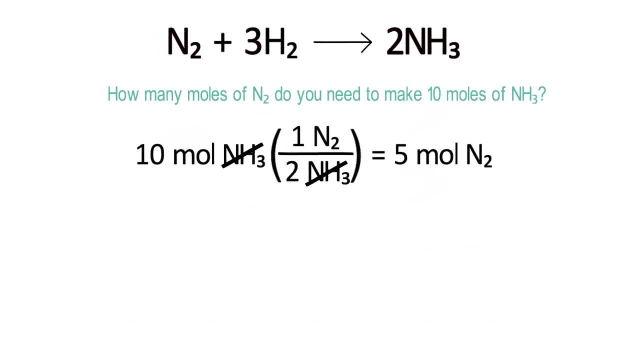 and we are left with moles of nitrogen, which is exactly what we want. Let's try one more problem: How many moles of ammonia can you make from 0.37 moles of hydrogen? First write down the quantity that you know. 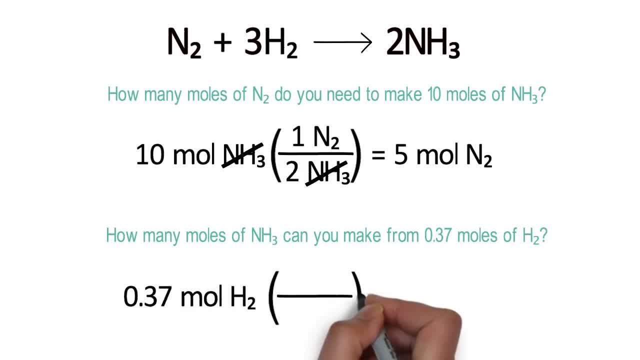 0.37 moles of hydrogen. Next, write a fraction and put three H2 in the bottom. The three H2 comes from the balanced reaction and the hydrogens cancel each other out. Then, because we are solving for ammonia, put two NH3 on the top. 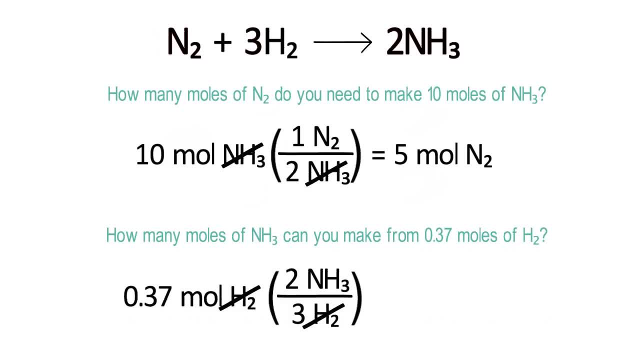 That two. NH3 also comes from the balanced reaction. Finally, do the multiplication in your calculator. If your calculator can't do fractions or doesn't have parentheses, simply multiply 0.37 times two and divide that number by three. The answer rounds to 0.25 moles of ammonia. 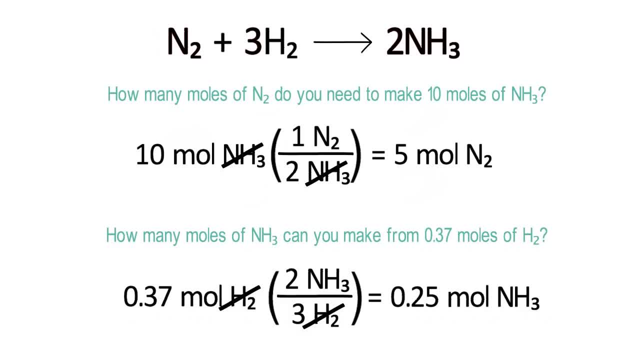 And that's it. Remember to always use quantities and moles when doing stoichiometry And remember that the balanced reaction is your conversion factor. Thanks for watching. If this video helped you at all, give me a thumbs up. I really do appreciate it. 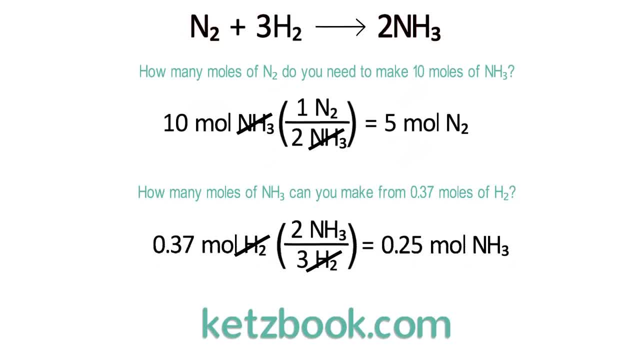 Feel free also to share any comments or questions you have below. subscribe to my channel or check me out at ketzbookcom.